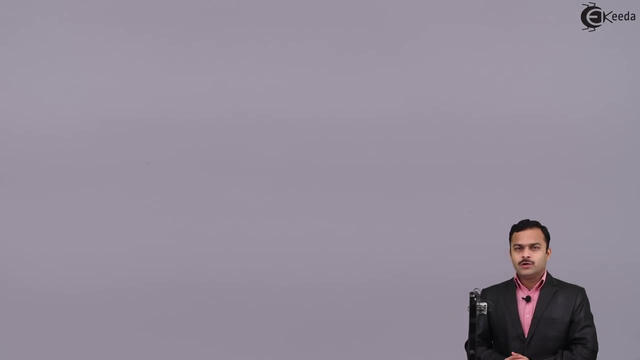 Hi, friends, in this video we are going to learn a concept of resonance in AC parallel circuit. Whether it is a parallel or series circuit, the concept of resonance remains same. And what is that? At resonance, the current taken by the circuit is always in phase with a voltage applied. 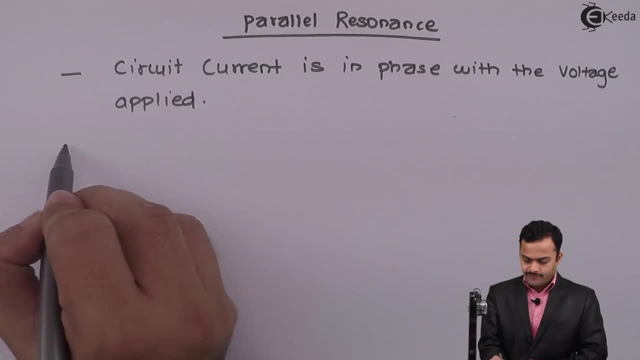 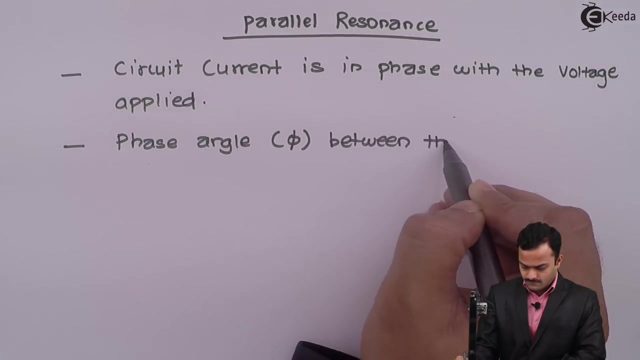 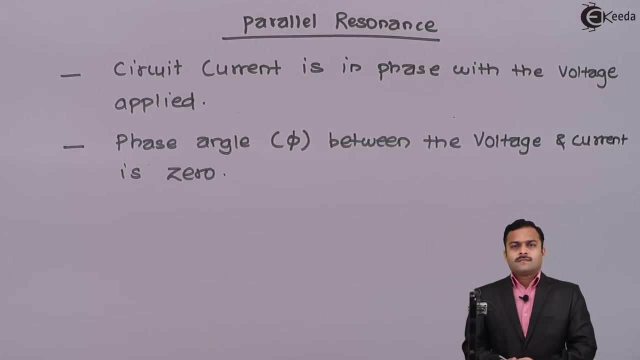 What is the meaning of in phase? In phase is nothing but phase. angle between voltage and current is zero. This is a property of resistive circuit. What does that mean? Despite of having inductor and capacitor in the circuit, at resonance circuit behave like a resistive circuit. 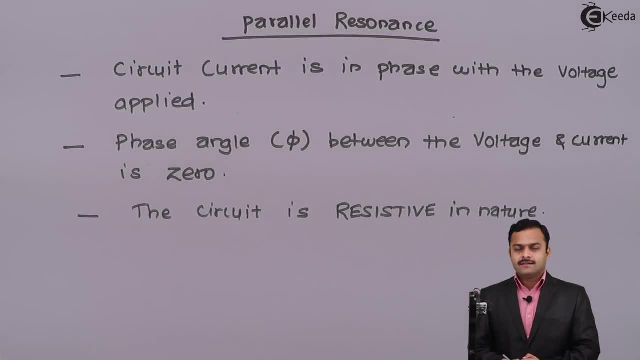 Being a zero phase angle, the power factor of the circuit will be unity. So these are the properties of any type of resonance. Now we are going to learn resonance with the help of a parallel circuit, which is more often we deal. So let's study that. 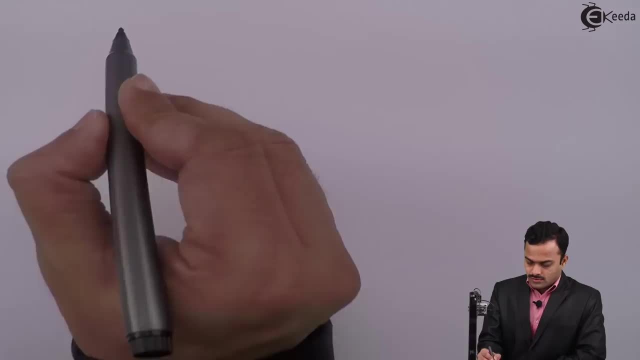 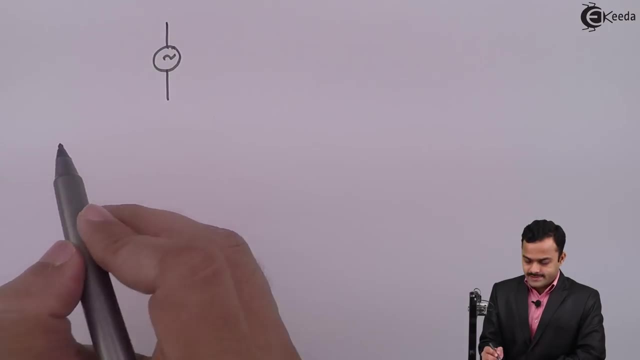 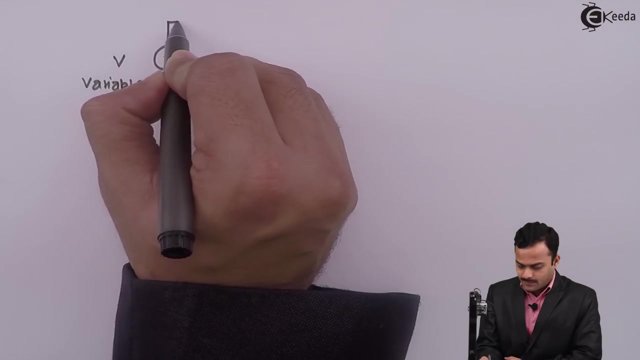 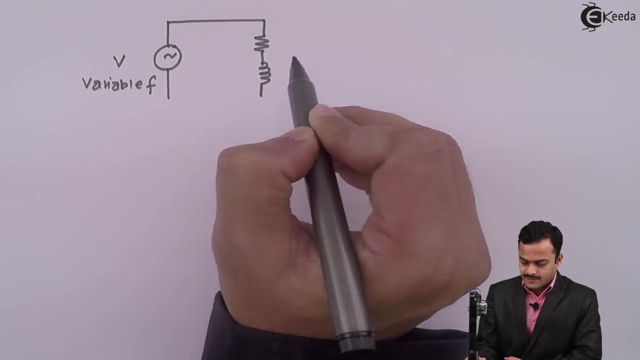 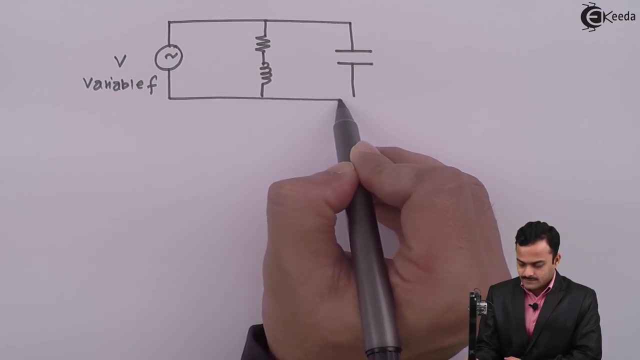 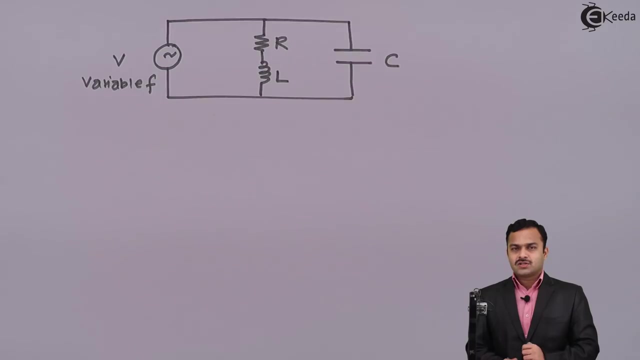 So I will have a voltage source with a variable frequency, Because resonance is a property or it is a function of a frequency. This AC supply is given to a circuit Having one practical coil connected parallel to the pure capacitor C. Now we are going to derive a expression of resonant frequency first. 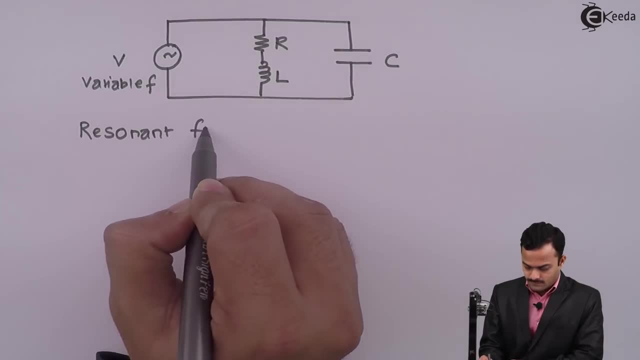 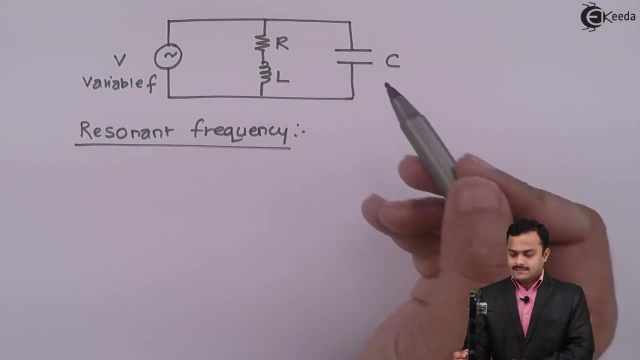 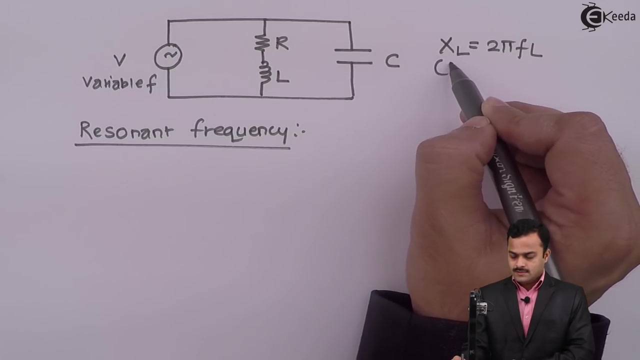 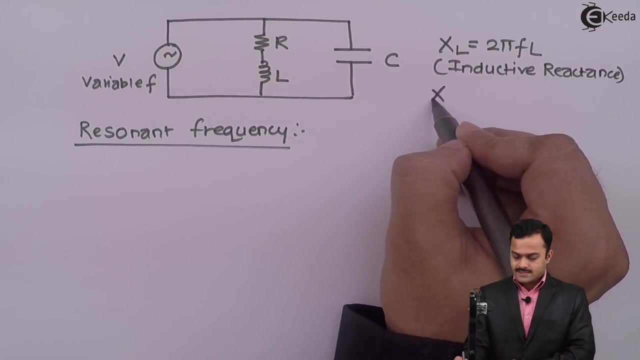 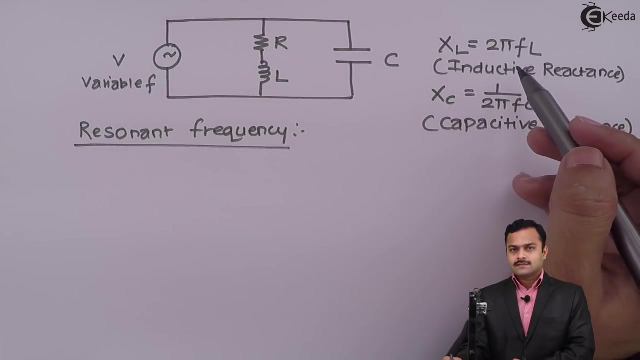 As we know, xL and xC is nothing but 2 pi fL, which we call as inductive reactance, And xC as 1 upon 2 pi fC, Capacitive reactance. xL and xC, both are the functions of frequency. 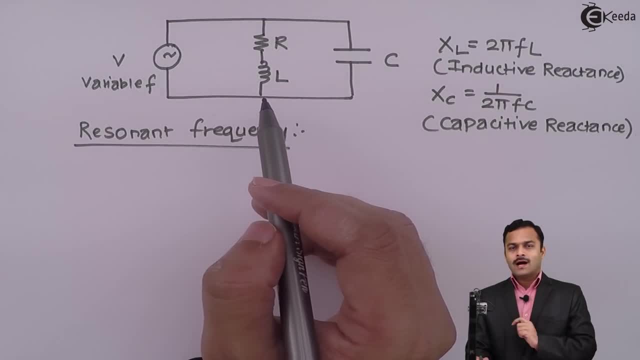 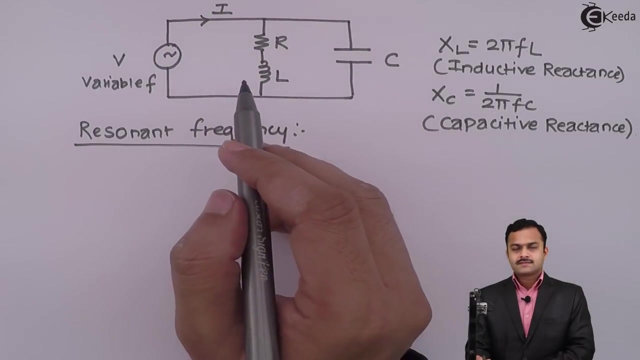 So therefore, you are having a variable frequency, And at one particular frequency the circuit behave like a resistive circuit. What does that mean? The phase angle between voltage and current is zero. So what we will do first, We will consider this as a branch number 1 and this as a branch number 2.. 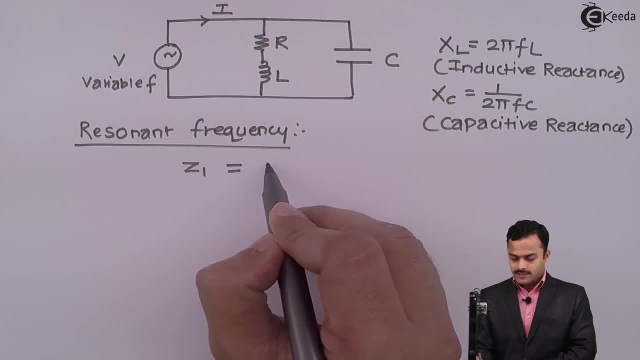 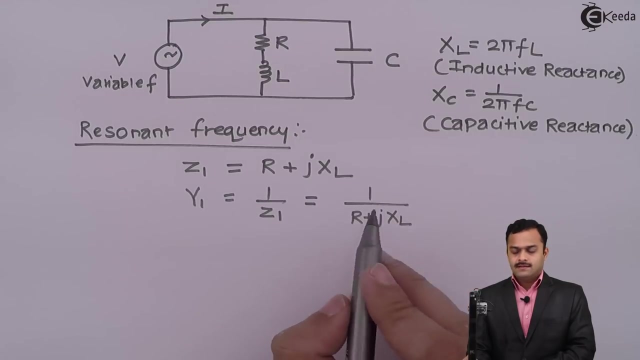 So for branch number 1, I will consider impedance z1 as R plus j xL. Its corresponding admittance y1 will be 1 upon z1.. So I substitute: I will get 1 upon R plus j xL. 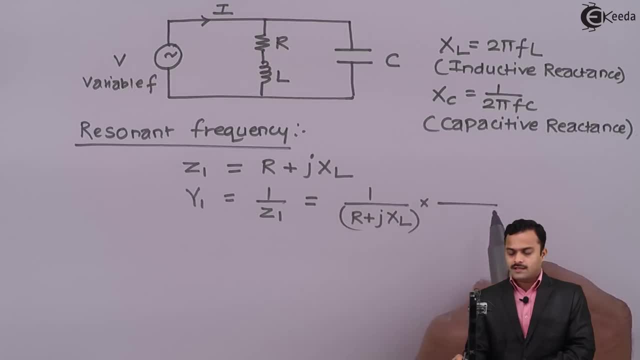 To get a proper complex number I will multiply and divide by complex conjugate, So R minus j xL getting multiplied as well as getting divided. So if I solve, I will get y1 as R minus j xL, R plus j xL, R minus j xL. 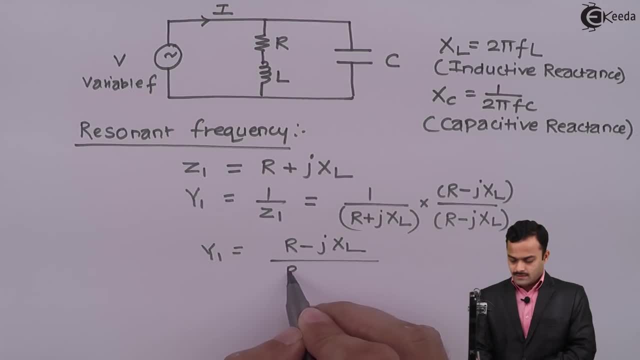 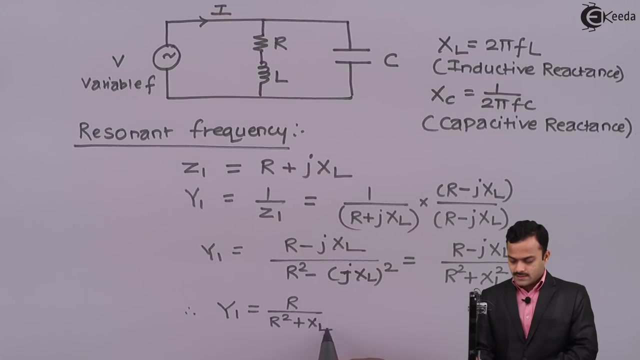 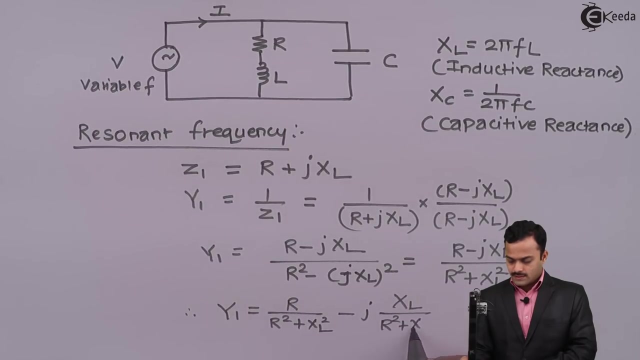 I will use a formula: a plus b a minus b, a square minus b square. So this will give me R minus j, xL upon R square plus xL square. So if I simplify, I will get y1 as R upon R square plus xL square minus j times xL upon R square plus xL square. 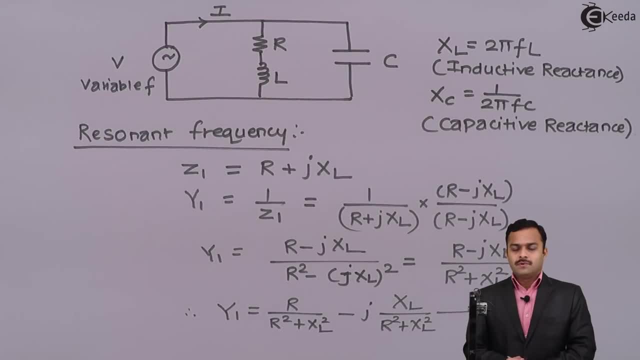 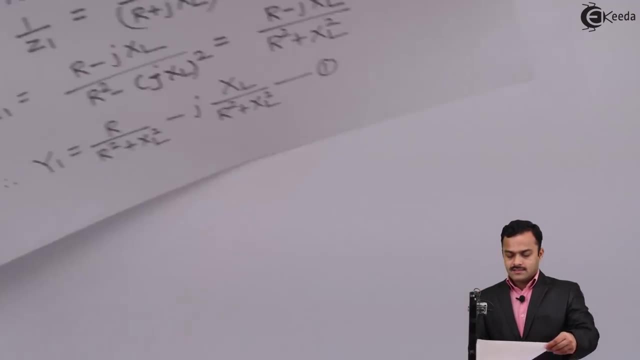 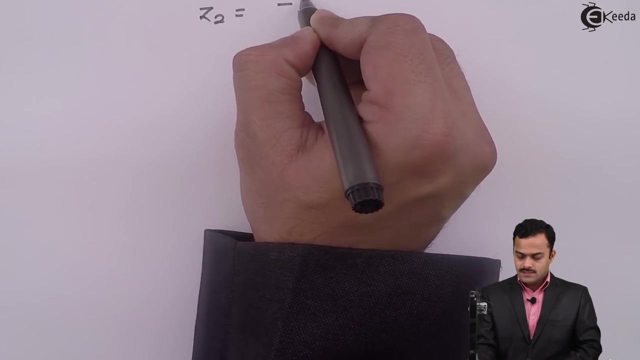 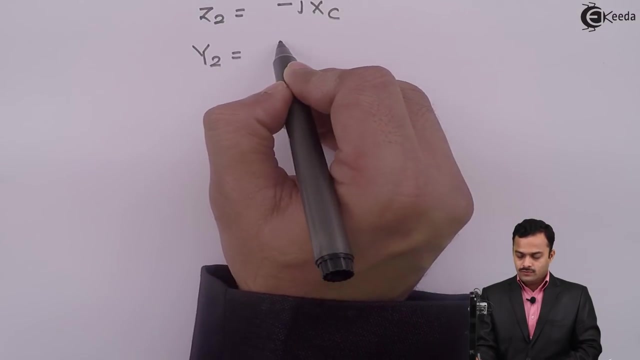 I will consider this as equation number 1.. Second branch is this: pure capacitance, So its impedance, z2 equal to minus j xC. So corresponding admittance: y2 equal to 1 upon z2 equal to 1 upon xC. 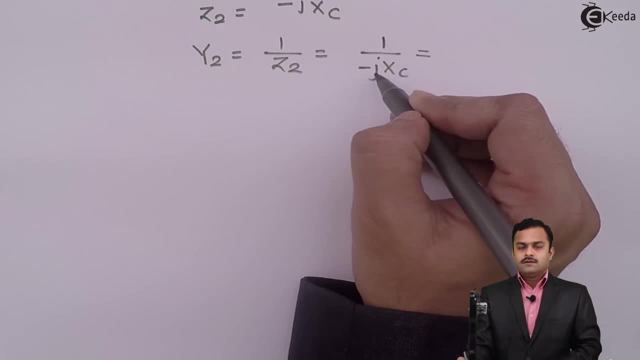 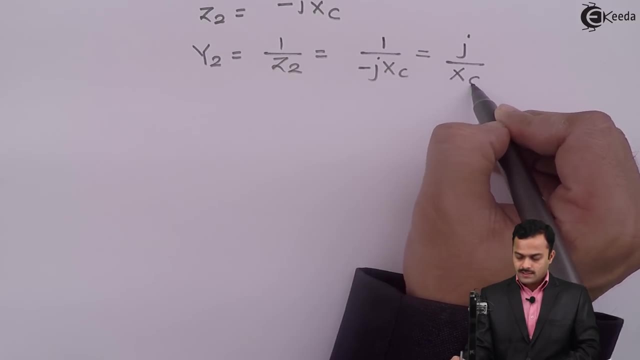 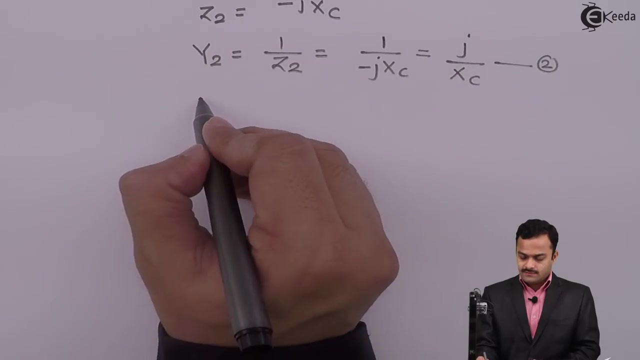 Minus j, xC. If I take this j up, this minus sign will go, So its j upon xC. equation number 2.. Now total admittance of the circuit will be nothing but addition of y1 and y2.. 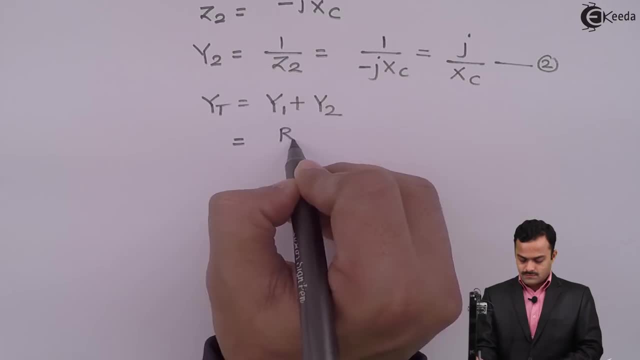 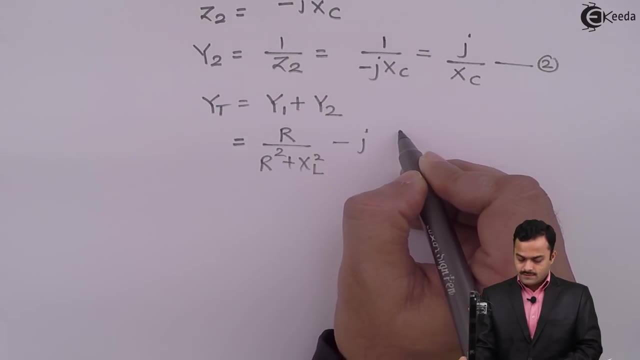 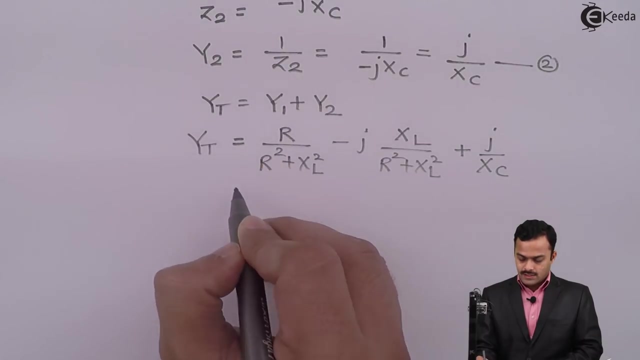 So y1 is R upon R square R square plus xL square, minus j, xL upon R square plus xL square plus j upon xC. So total admittance is also a complex number with a real term: R upon R square plus xL square. 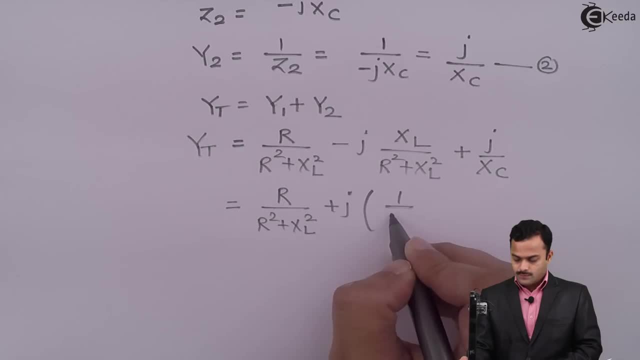 And imaginary part is 1 upon xC minus xL upon R square plus xL square. Now, at resonance circuit behave like a resistive circuit. That means imaginary part of impedance or imaginary part of total admittance equal to 0.. 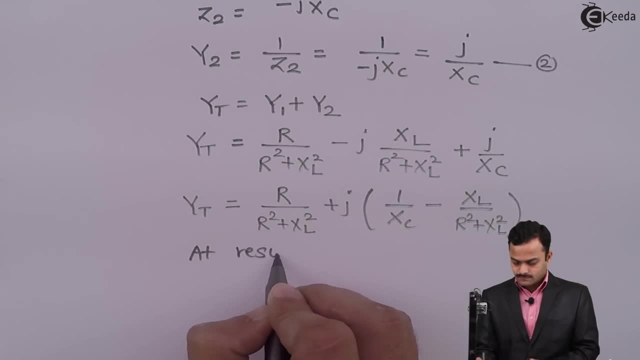 So at resonance imaginary part of yt is 0. So if I consider the imaginary part of yt is 0. That means I have to equate this part to 0. So if I do that, what I will get? 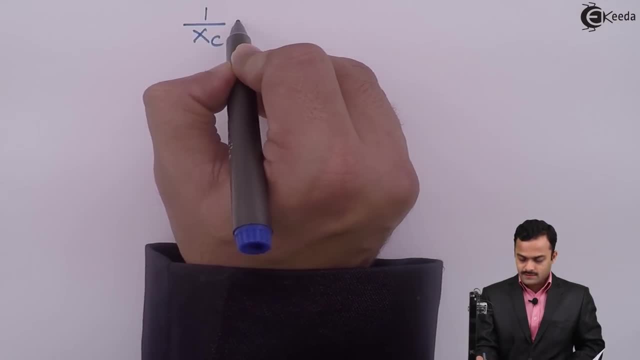 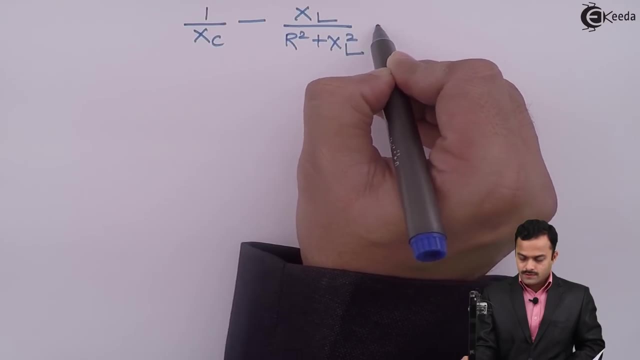 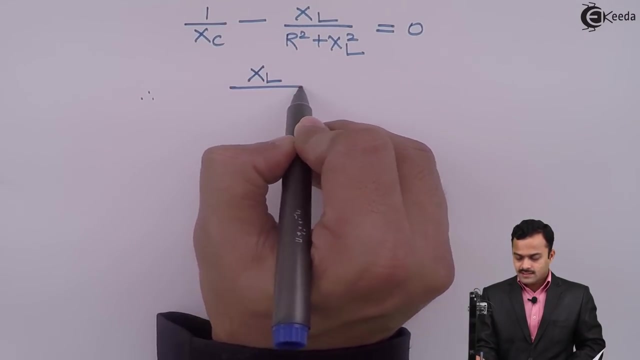 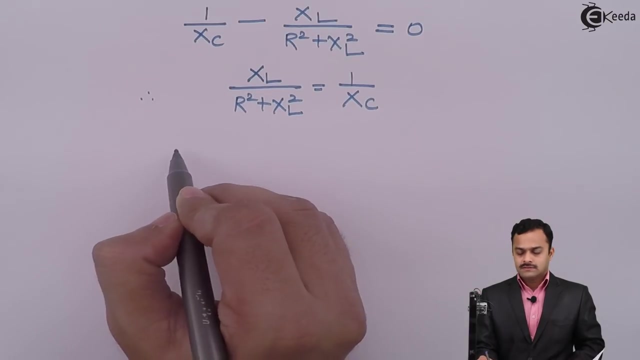 1 upon xC minus xL upon R square plus xL square, equal to 0.. So if I simplify further, I will get xL upon R square plus xL square equal to 1 upon xC. Let us cross multiply. 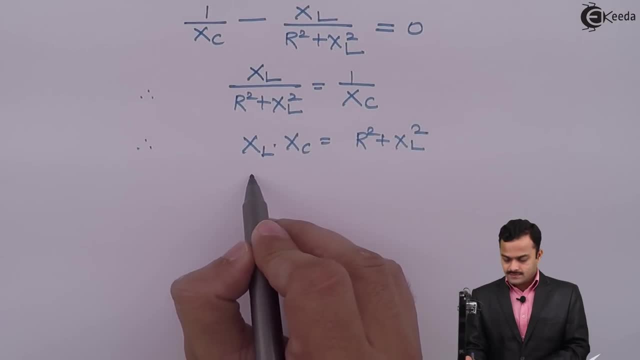 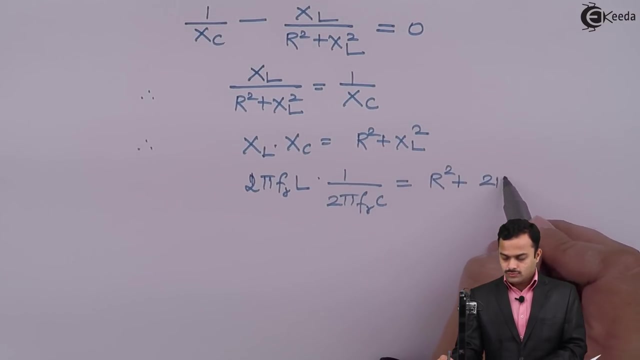 So if I substitute xL as 2 pi F R L, Why F R? Because this particular phenomena is appearing only when F equal to F R And x is 1 upon 2 pi F R, C equal to R square plus 2 pi F R L whole square. 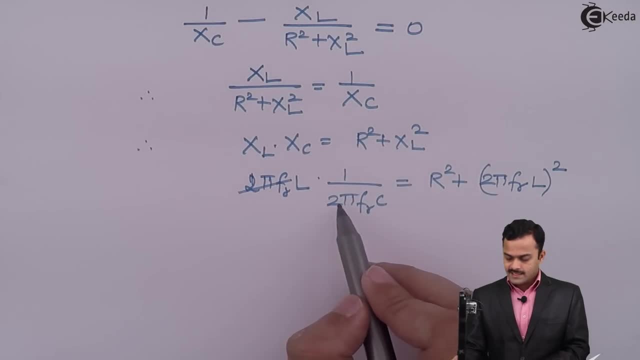 So 2 pi F R get cancelled. I will get L by C equal to R square plus 4 pi square, F? R square L square. Remember I need to get expression of F? R. So I will keep 4 pi square L square multiplied by F? R square on this side. 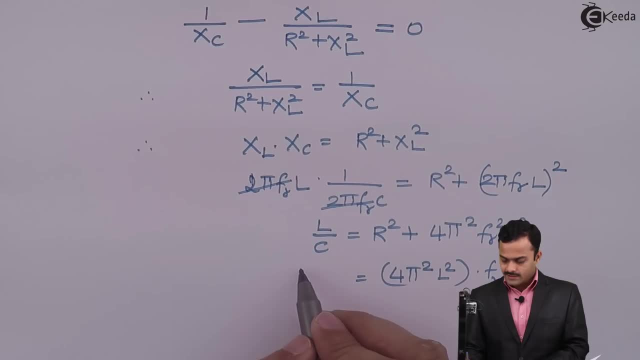 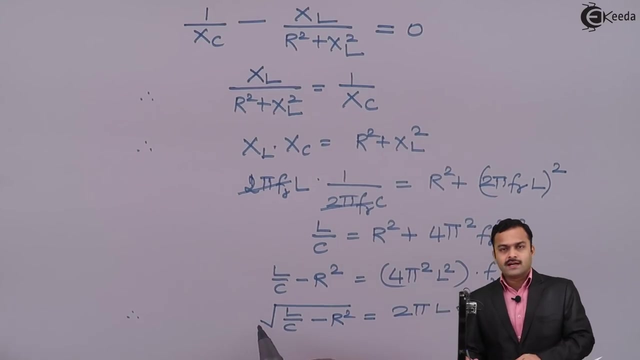 And here I will have L C minus R square. So if I take the root, I will get root of L C minus R square equal to 2 pi L F? R. Let us take this 2 pi L over here in order to get F? R. 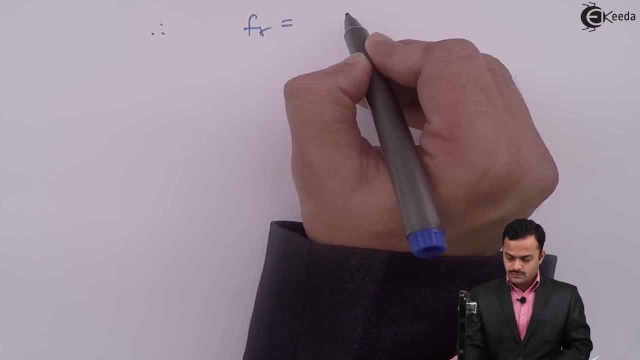 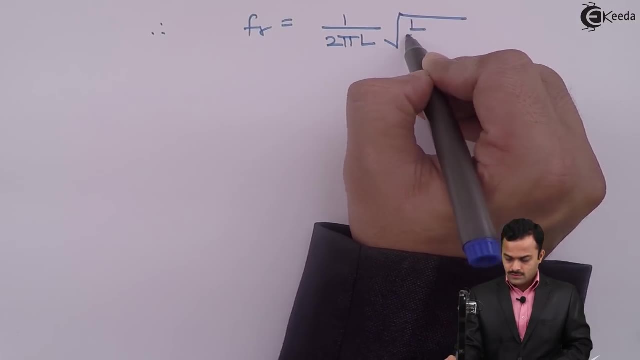 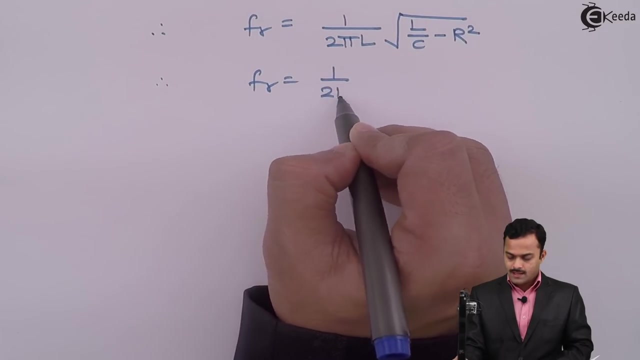 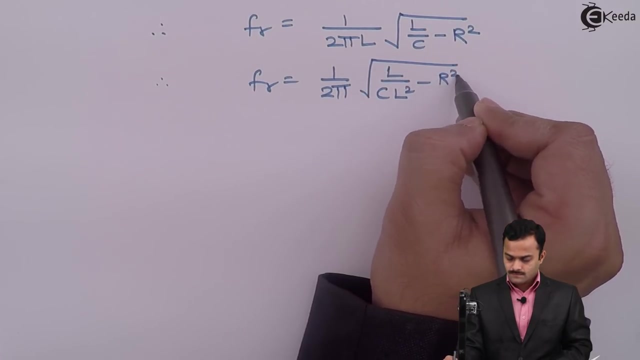 So F? R equal to 1 upon 2 pi L under root L by C minus R square. Let us rearrange the term properly Meaning. I will take this L inside a root, So it will become L square. So after simplifying I will get: F? R is 2 pi L. 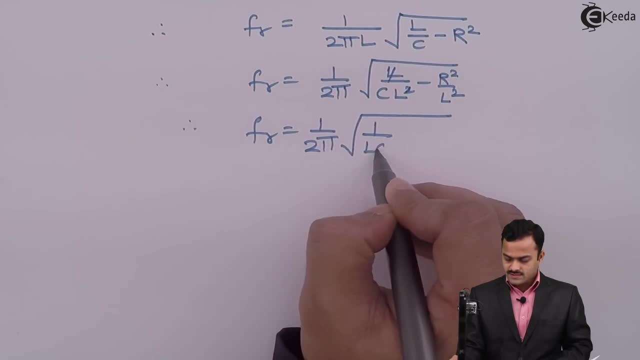 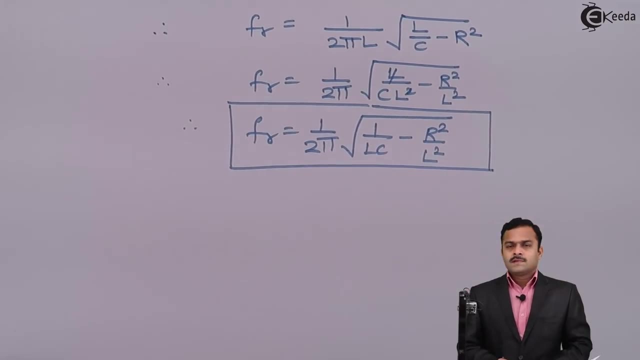 So F? R is 2 pi root of 1 by L C, minus R square by L square. So this is the expression of resonant frequency I will get at which the circuit behave like a resistive circuit. Let us find out its resistance, which we call as dynamic resistance. 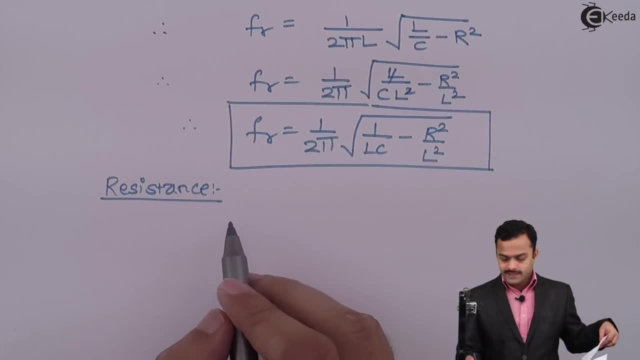 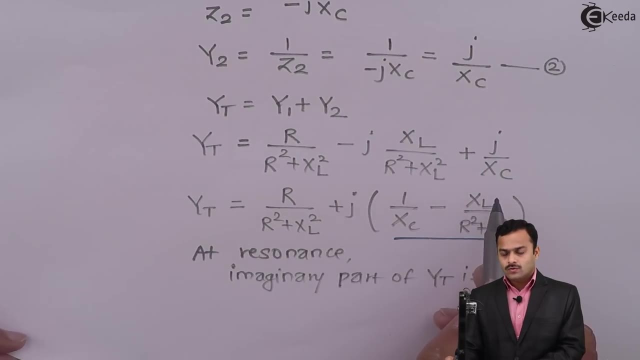 So for that purpose, let us go back to y t once again. So y t is like this: At resonance, this term is becoming 0.. So at resonance, y t is nothing but R upon R square plus x, L square. 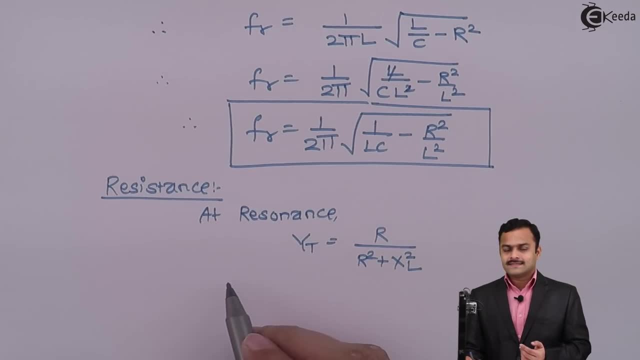 This is the admittance. We want resistance or impedance, you can say So that we call as a dynamic resistance. So that is 1 upon y t. The answer you will get is R square plus x, L square upon R. So the dynamic resistance or impedance is R square plus x, L square by R. 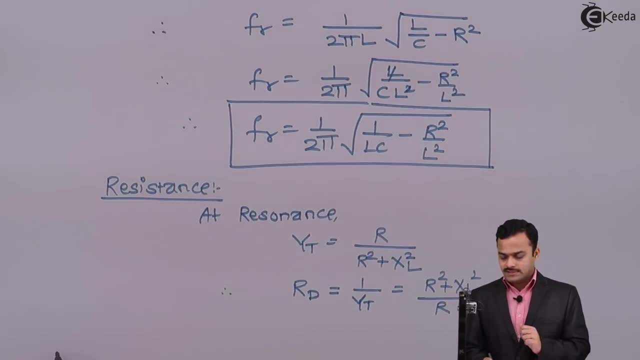 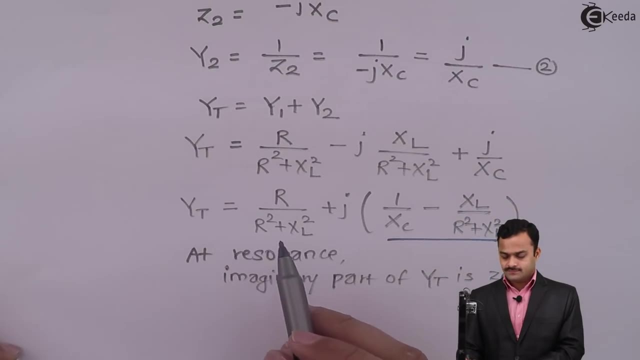 Let us check What exactly happening at resonance, especially a parallel circuit, is concerned. So once again I will go to y t expression. So what is happening over here? y t is given by this expression and at resonance this term is vanishing. 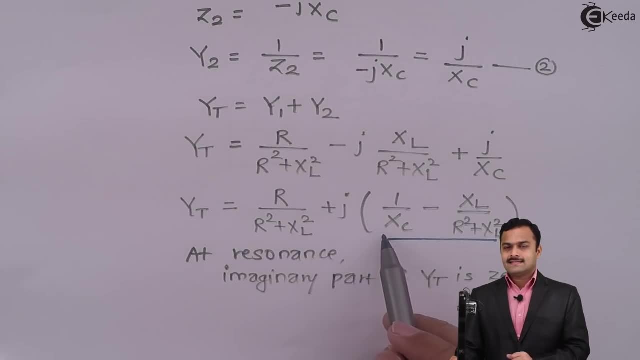 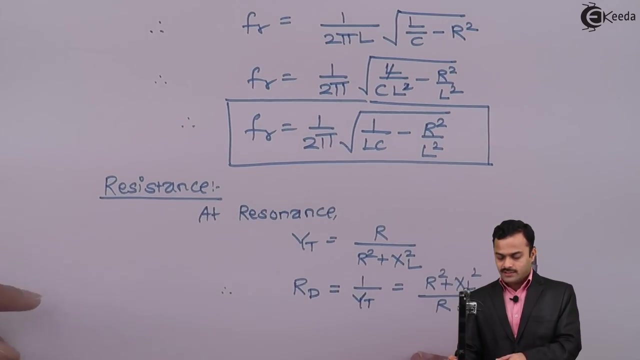 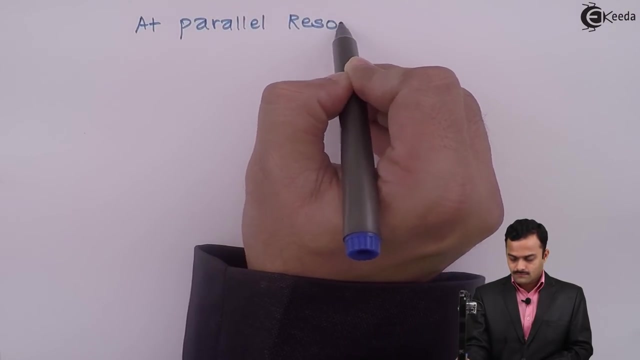 So what is happening? y? t is decreasing, y? t is decreasing. What does that mean? That means impedance is increasing. at parallel resonance- This is a very important conclusion we get, So I will write over here: At parallel resonance, admittance decreasing. 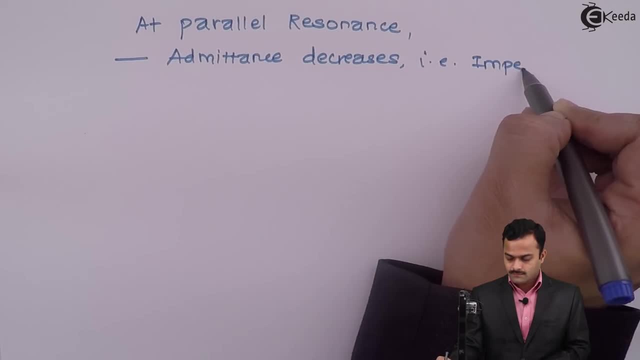 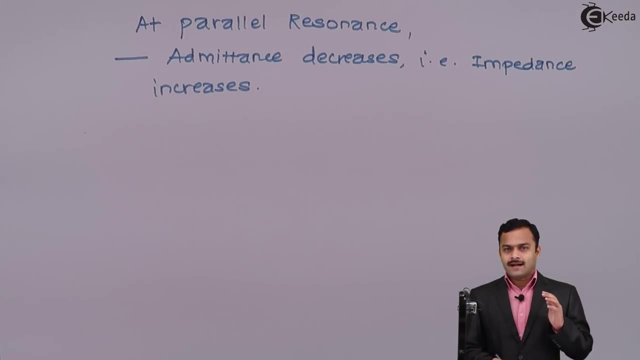 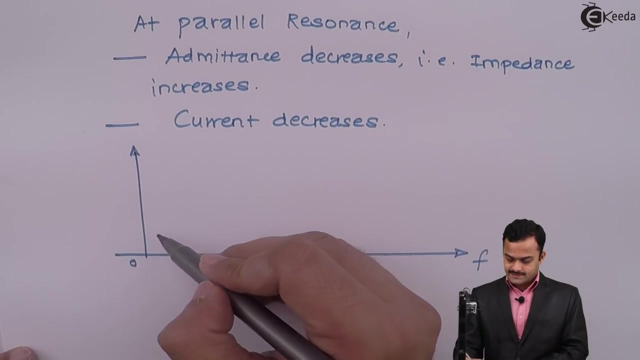 That is, impedance increases. If impedance increases, obviously current drops. So if I draw the nature of current and impedance against the frequency, It will be like this: Impedance increases. So at resonance you will have a maximum value of z.